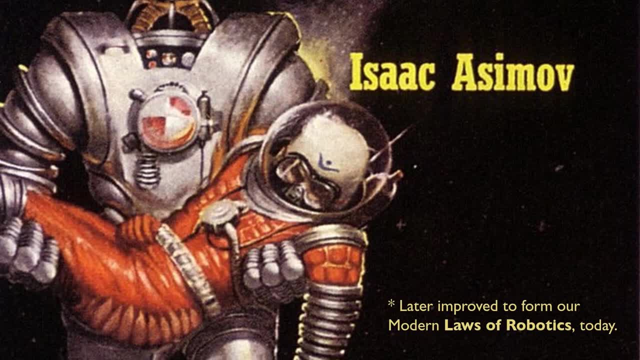 concepts of artificial servants or soldiers date at least as far back as the ancient legends and mythologies. And if I talked about every little step or advancement of this robots, you'd probably have to sit here all day. So I'll try to put it as simple as possible. 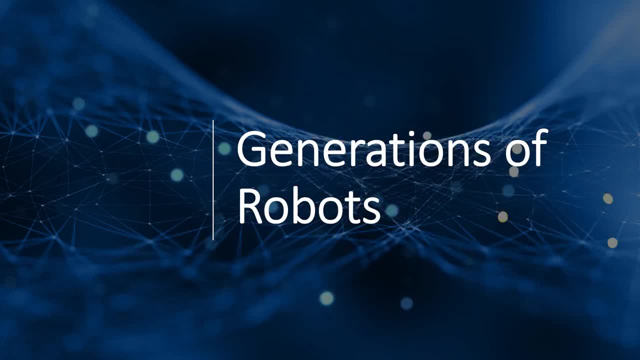 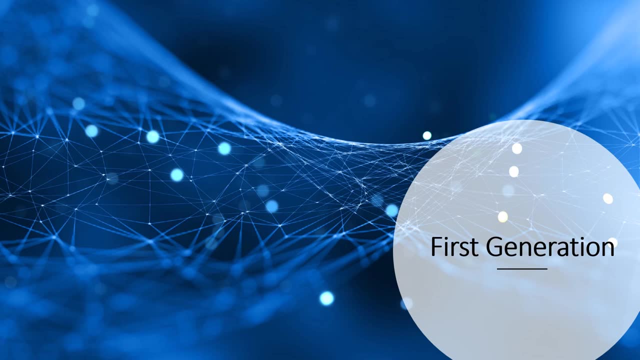 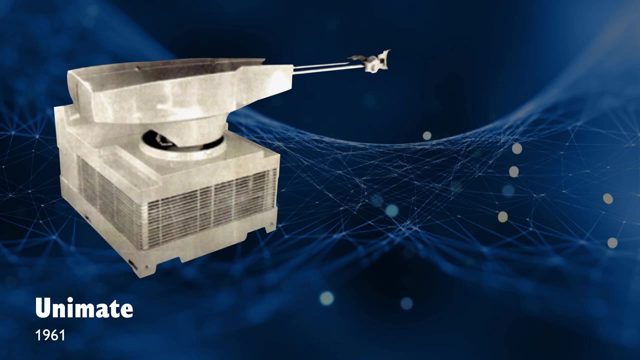 So what I've done here is I've segregated this into various generations. So I think the industry is a good place to start, Because that's where robots originally started to add purpose. Since factory work can be repetitive and requires quite heavy lifting, it's ideal to employ robots in this domain. 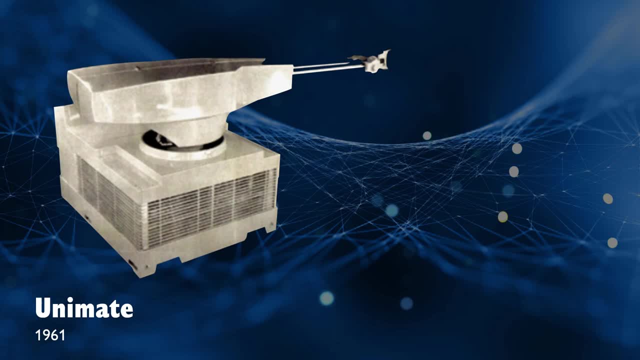 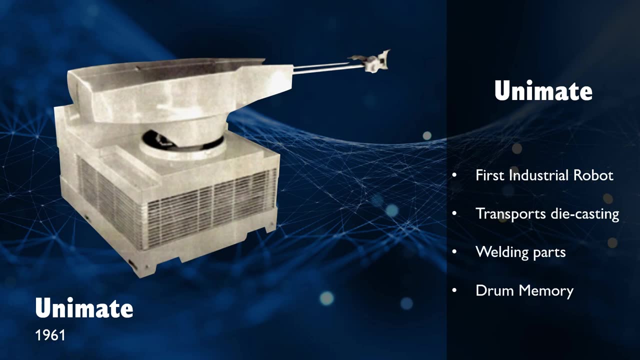 The world's first industrial robot, Unimate, was installed in a General Motors production line in New Jersey 1961.. The original Unimate consisted of a large computer-like box joined with another box which was connected to an arm. It had systematic tasks stored in a huge 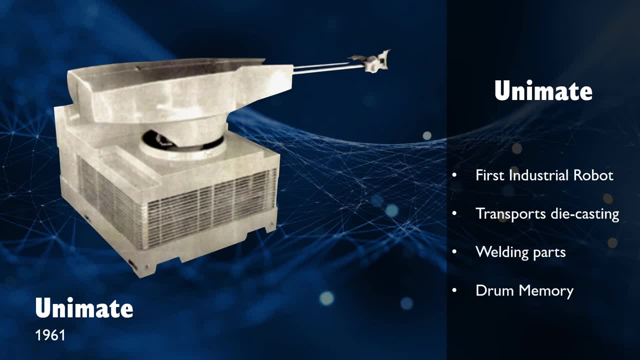 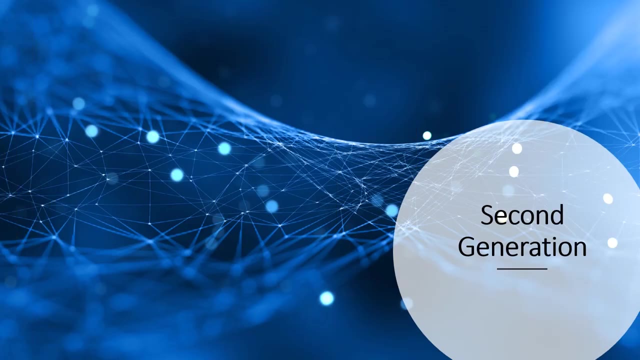 magnetic drum. The machine undertook the job of transporting die castings from an assembly line and welding these parts into autobodies- A dangerous task for workers, who might be poisoned by the toxic fumes or lose a limb if they were not careful enough. 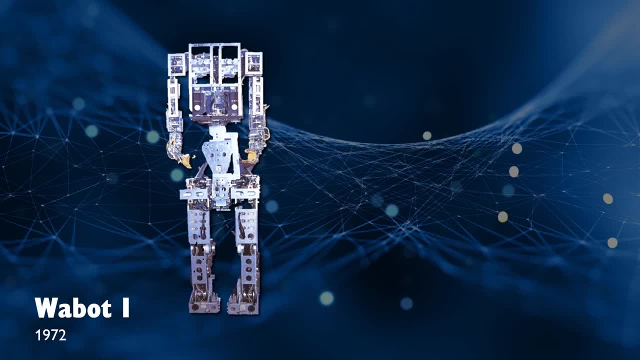 From then on, Japanese robots have led the field. Waseda University initiated the Vobot project in 1967, and in 1971, the Vobot project was launched. The Vobot project was launched in 1967, and in 1971, the Vobot project was launched in. 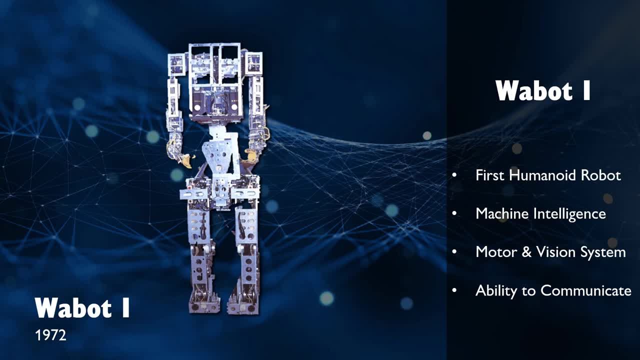 1972, completed the Vobot-1, the world's first full-scale humanoid intelligent robot. Its limb control system allowed it to walk with lower limbs and to grip and transport objects with hands using tactile sensors. Its vision system allowed it to measure distances. 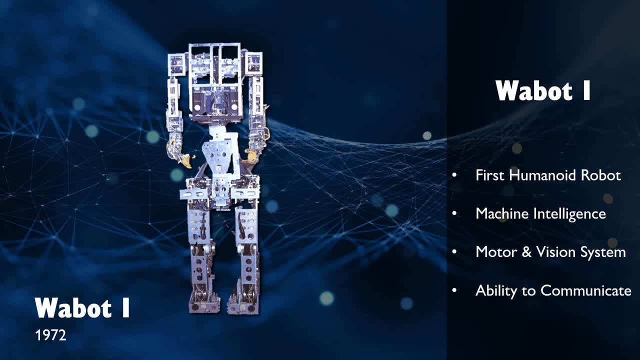 and directions to objects Using external receptors, artificial eyes and ears. it was the best of its time, And it could also converse in Japanese with people Using a conversation system and an artificial mouth. this was truly the world's first android- Android being man-like, and it truly lived up to its meaning. 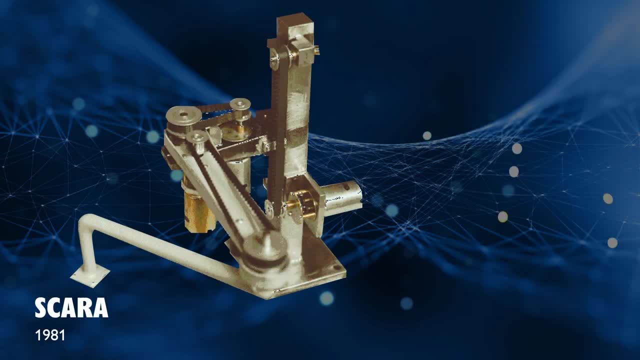 Another bot from this generation is the SCARA, or the SCARA. This acronym stands for Selective Compliance Assembly Robot Arm. By virtue, it's only an arm which was rigid in the Z axis and pliable in the X and Y. The jointed two-link arm layout was designed to allow the robot to move freely and easily. 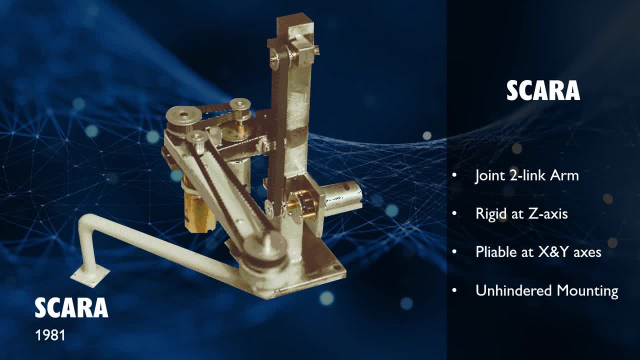 The robot was designed to move freely and easily. The robot was designed to move freely and easily. The robot is the closest we could get that time to our human arms. It was quite beneficial in the transferring domain, where it could transfer parts from one cell to another. 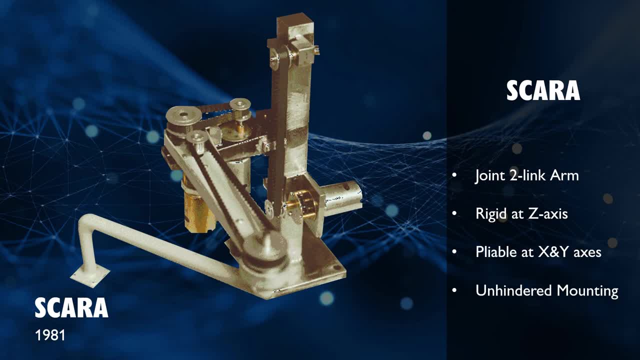 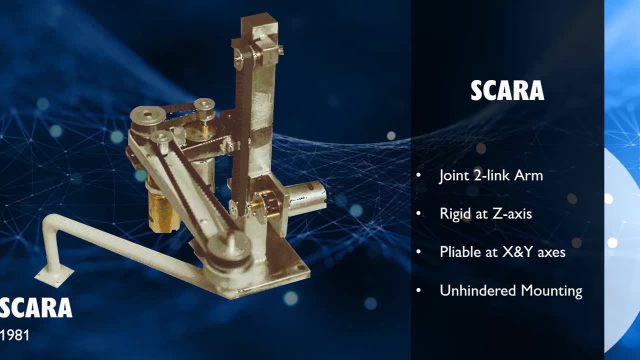 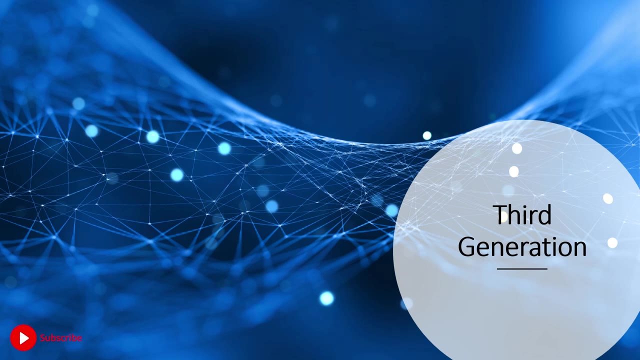 or for loading and unloading processes. To be honest, really, it's a beautiful invention for lazy people like me, else I wouldn't even get up for the TV remote myself. Moving on, we have the 3rd generation Now. the 3rd generation did not have a TV remote. 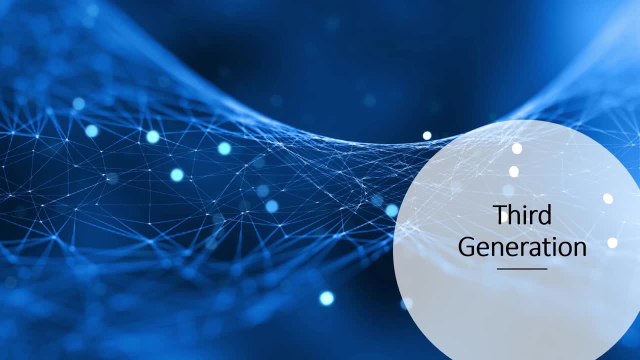 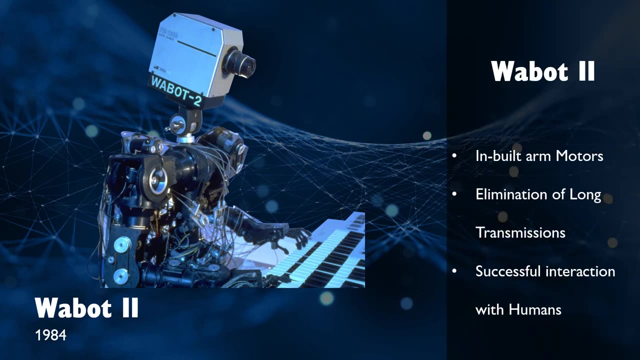 nor did it have much of a leap, but boy oh boy, did it take the world by storm when it did, Presenting to you Vobot 2, the musical robot. This bot could not only read musical score but also play, thanks to its inbuilt motors in the arms, With its visual and vocal subsystems. 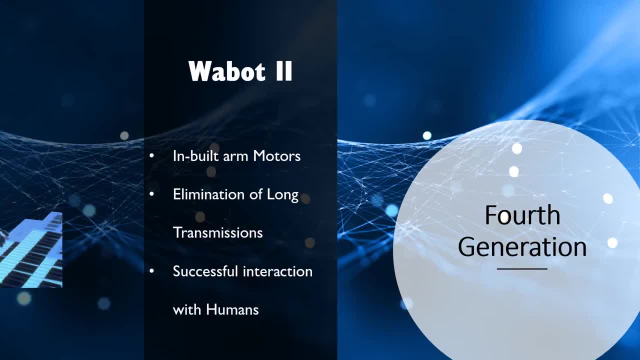 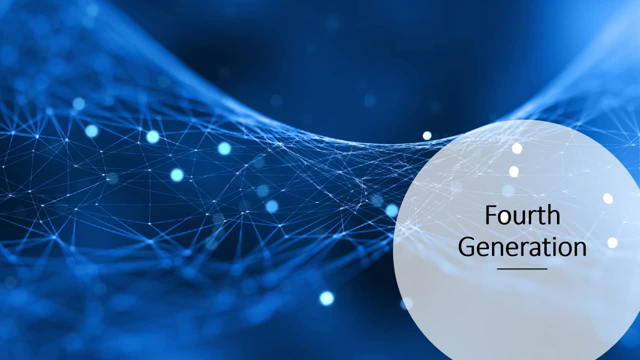 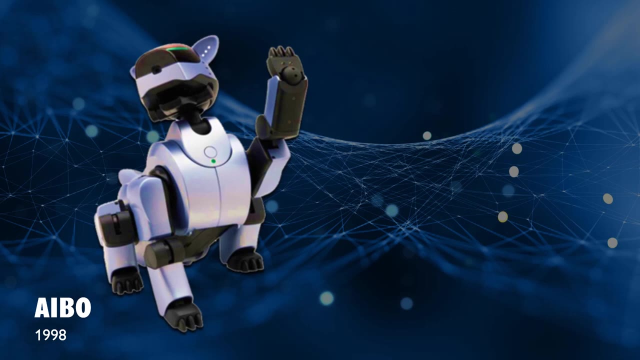 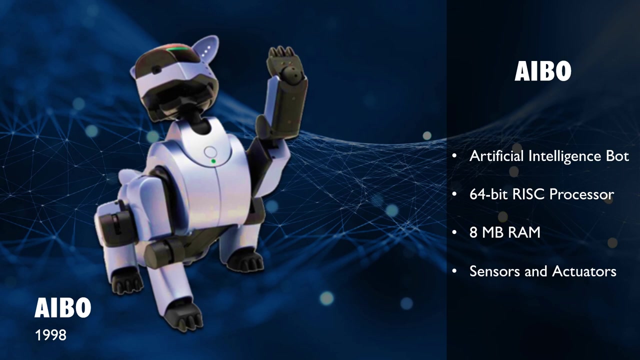 it could successfully hold conversation as well. With that we move to Gen 4. And the first of its kind, Artificial Intelligent Robots, or the AIBO, which is a part of a series of robotic pets designed and manufactured by Sony, having actuators for life-like movements. 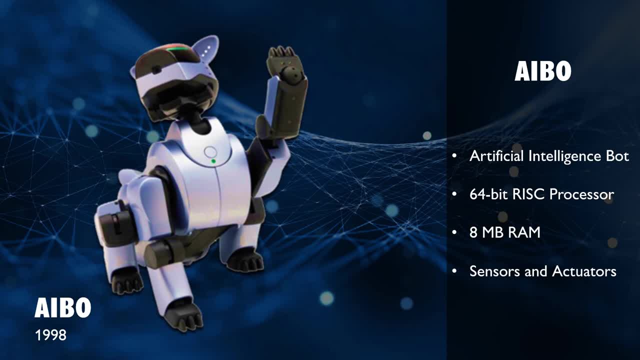 in its legs, neck and tail. Imagine having a pet, but none of the dirty work, isn't it a dream? With sensors to enable touch sight, range-finding and actual dog-like speed? this one's a keeper. So what is Gen 4?? 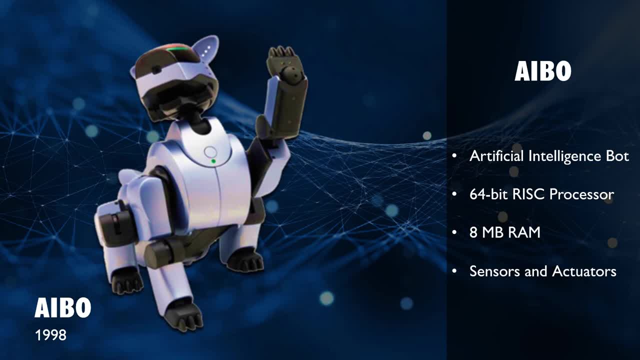 2017, Sony announced a new generation of AIBO after almost 11 years. They promise that this one is going to be more dog-like than ever. I can't really wait for its reveal, can you? So, with that said, let's move to another bot in this generation, where the artificial 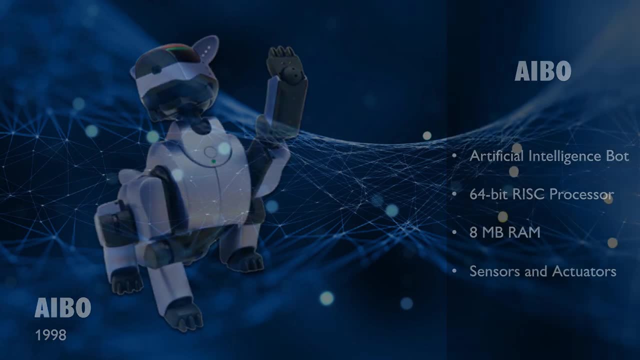 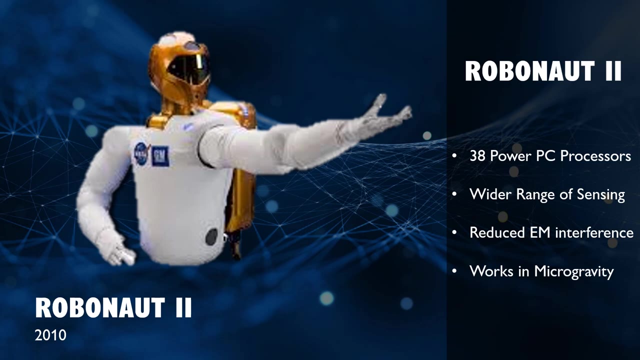 intelligence really shines through. Originally designed to test how machines work in microgravity, this one outshone its predecessors with a wider range of sensing, reduced flammability and reduced electromagnetic interference. it is the perfect space help for the International Space Station. According to experts, any robot of a sort yet to be seriously put into operation. 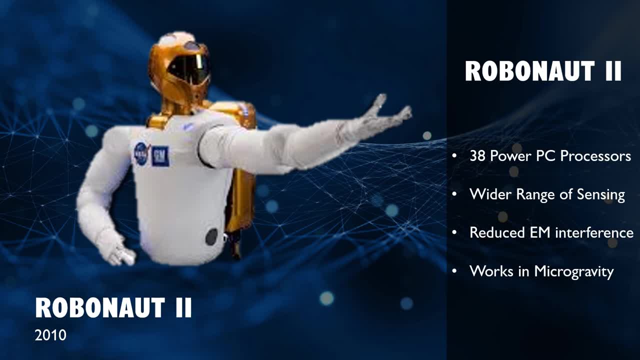 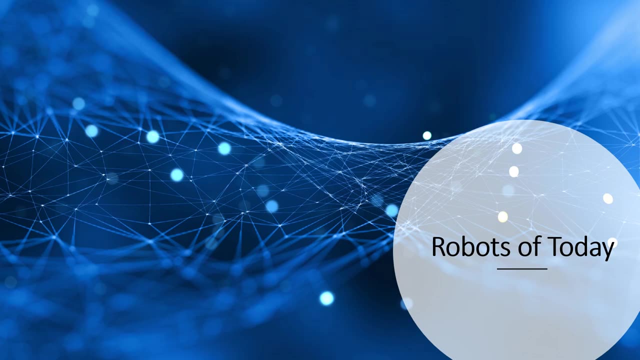 is a 4th generation robot. Examples of these might include robots that reproduce and evolve, or those that incorporate biological as well as machines, mechanical components. past that, we might say that a fifth generation robot is something that nobody has designed, but there is still a robot i would like to talk about that brings the world's 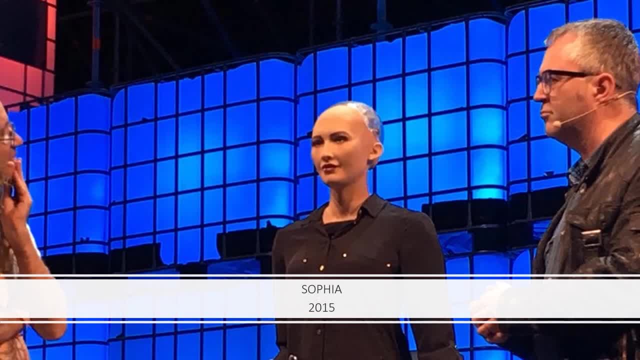 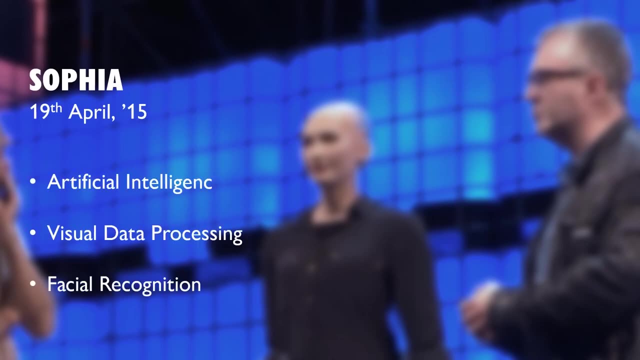 tomorrow to its today. this is sofia, the robot celebrity mostly known for her human-like appearance and behavior. compared to its previous robotic variants, sofia uses artificial intelligence, visual data processing and facial recognition. sofia also imitates human gestures and facial expressions. she herself is capable of more than 200 different facial expressions. she can even 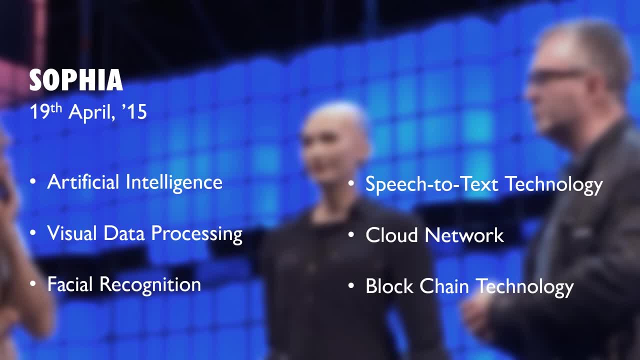 answer certain questions and make simple conversation on predefined topics. sofia uses speech-to-text technology and is designed to get smarter over time. the information is shared in a cloud network which allows input and responses to be analyzed in a blockchain technology. she was designed predominantly to help the elderly in nursing homes. so with that i conclude my list of generations of. 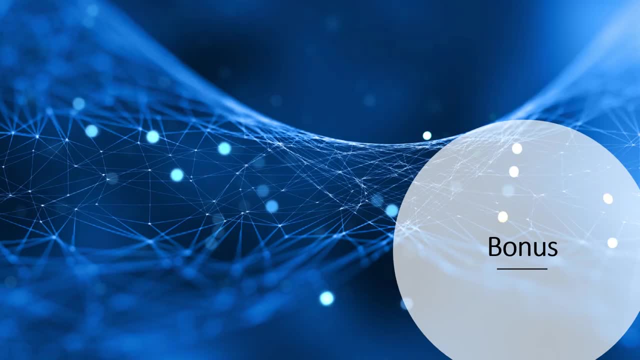 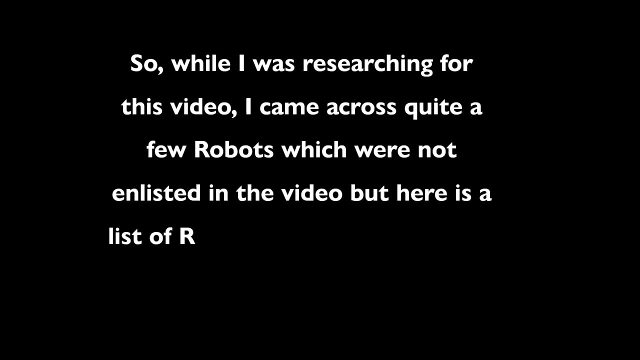 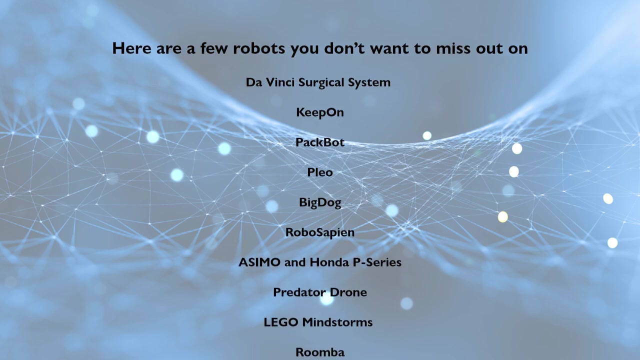 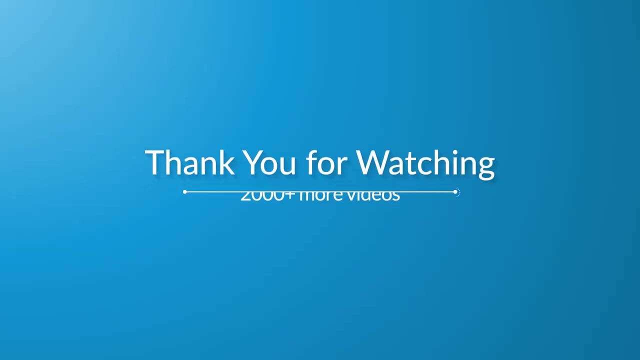 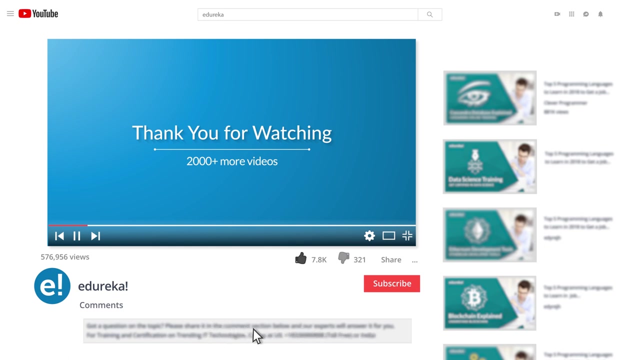 robots. which one did you find most revolutionary? leave a comment below to let us know. thank you and have a great day. i hope you have enjoyed listening to this video. please be kind enough to like it and you can comment any of your doubts and queries and we will reply them to you. 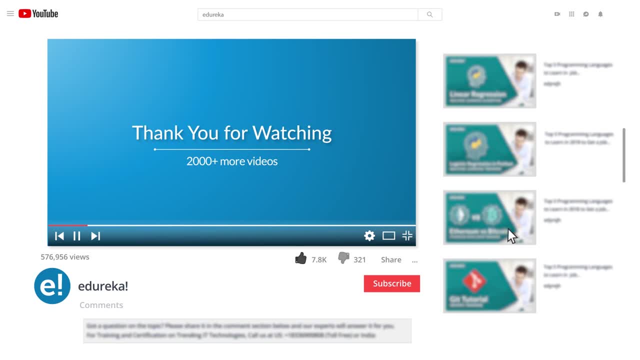 at the earliest. do look out for more videos in our playlist and subscribe to edureka channel to learn more happy learning.